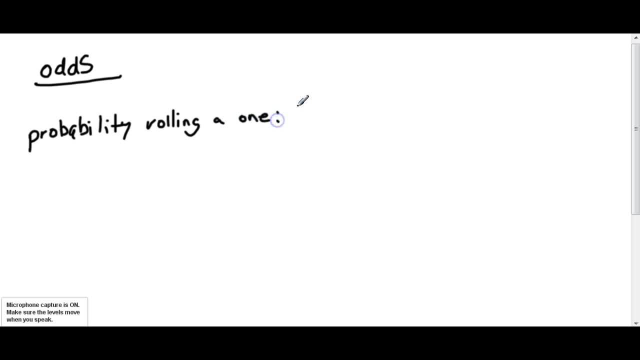 So the probability of rolling a 1 with a dice- And we're going to talk about probability- is: we know that there's six numbers on a dice and there's only one, 1, so the probability is 1 out of 6.. Okay, that's the probability of rolling a 1 on a regular dice: 1 in 6.. Okay, 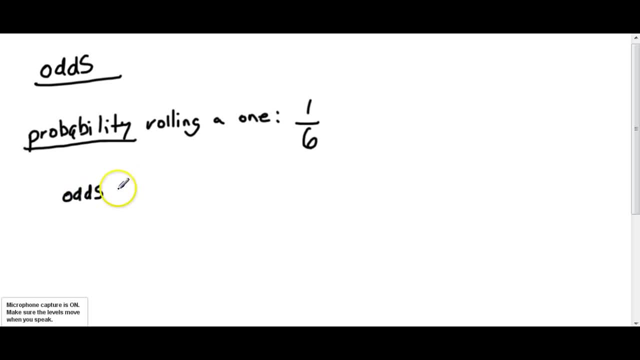 Odds, however, are something a little different. Odds are just a comparison of the favorable outcomes versus unfavorable outcomes, So let's take the standard six-sided dice. here We want to say: well, we know, the probability of rolling a 1 is 1 out of 6, but what are the odds of rolling a 1?? 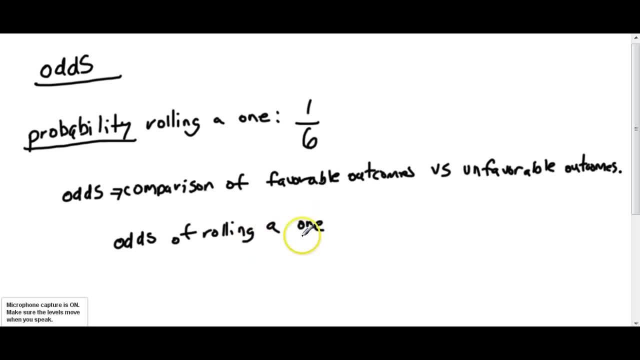 Okay. well, the odds of rolling a 1 are just the favorable outcomes 1,, 2,, 3,, 4,, 5,, 6, 6.. Compared to the unfavorable outcomes 1,, 2,, 3,, 4,, 5, 6.. 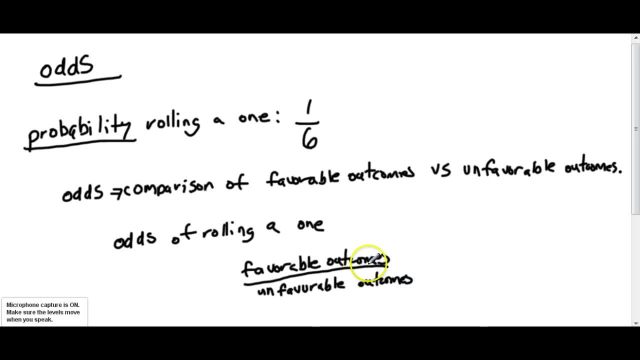 Okay. So the favorable outcomes in rolling a 1 on a dice is well, is 1.. And the unfavorable outcomes is not 6, because 1 is included in the 6.. If you're not sure that there's a 1 in in a dice, you know that there is a 1.. 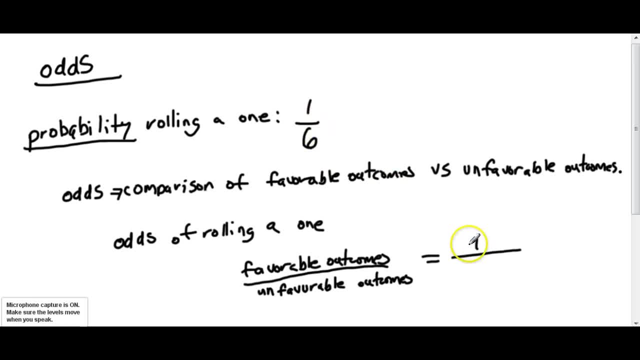 in the six. if you're not going to roll a one, you're going to roll a two, three, four, five or six, which is the five other numbers. okay, so odds of rolling a one are favorable, which is one chance or one shot, compared to the unfavorable outcomes of rolling one, which is five against. so, basically, 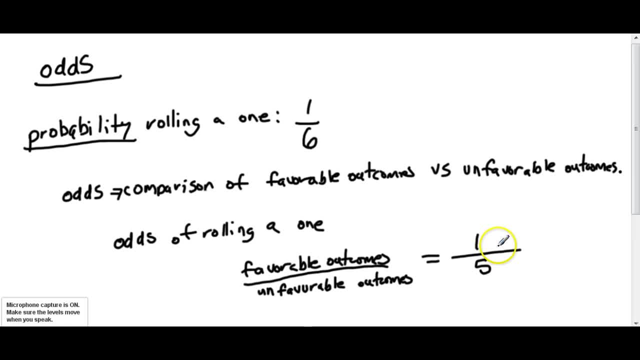 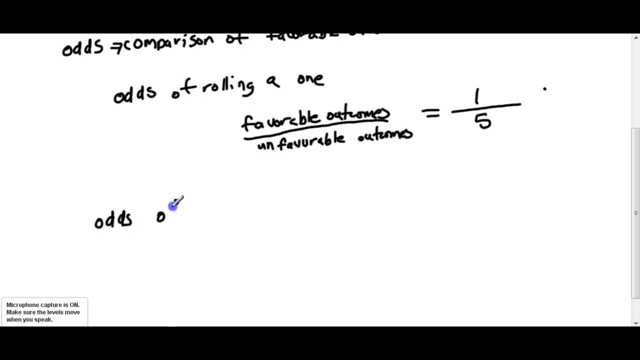 it's one, four and five against. so that's odds expressed as a fraction, but usually odds are expressed as a ratio. so we would say that the odds of- let me just move this down here a bit- the odds of rolling a one is one to five. okay, this would be odds in favor of rolling a one. the odds. 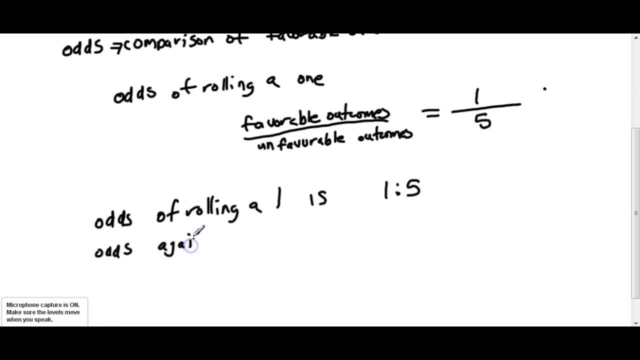 therefore against one, we can see. the odds against rolling a one is just the reverse. you've got five other chances to roll another number- two, three, four, five or six- compared to the one, so it would just be reversed. the odds against is just five to one. okay, so 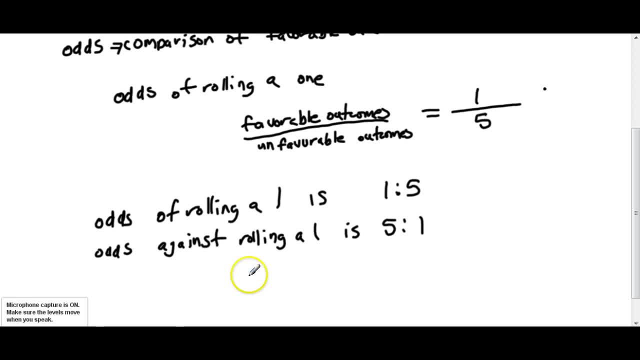 basically, in a nutshell, odds is a very simple concept. it's just basically a ratio, okay, and this is a ratio that compares a two to one chance to roll another number: two, three, four, five or six. the desired events to the number of undesired events, or vice versa. 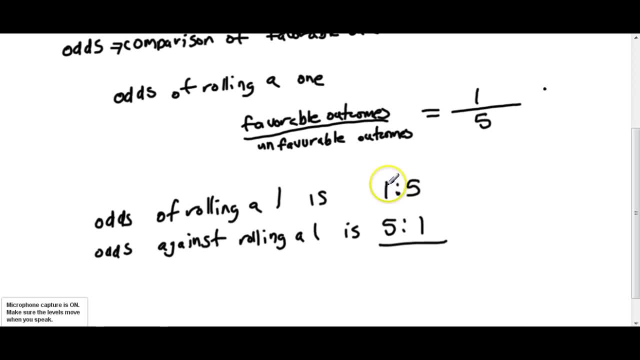 so in this case the desired event is to roll a one. so we have a one-in-five chance or one in five odds of rolling a one, and the odds against rolling a one is five to one. okay, so can be favorable versus unfavorable or unfavorable versus favorable. it can be. either one. okay, so just your mile or distance, verk. It is only possible if you always follow the formula. if it's only possible, a single loss or a hit, isин one with an advantage idee, bring down above this crispy. okay, SO it can be favor Меня. 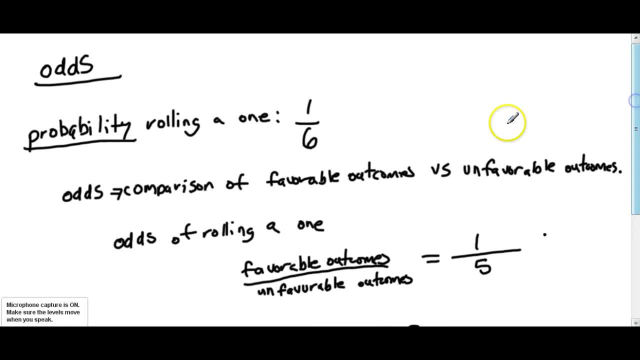 engines. as I said back there, It is only possible if you always follow the formula. if using multiple strategies, other factors are not appropriate, very often yougn. So just remember that there is a difference between probability and odds. Probability is a comparison of a chance compared to the total number of chances. 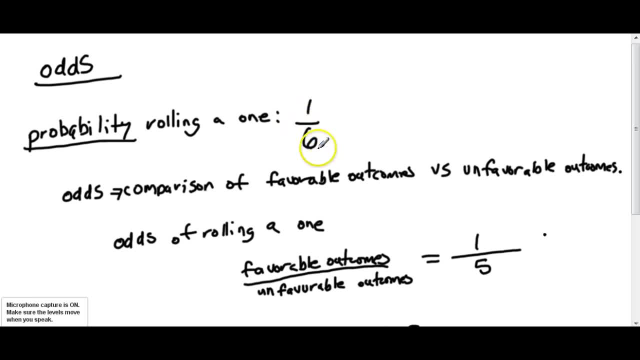 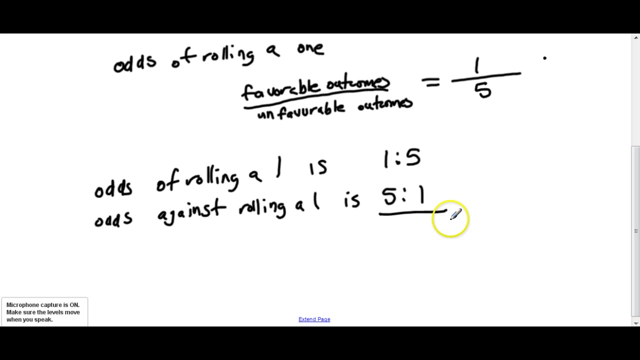 So rolling a one out of a total of six Odds, however, is favorable versus unfavorable, or unfavorable versus favorable, and it is rolling a one compared to the other numbers, excluding the one. So you can see the difference there. Alright, so go ahead and work in your workbook.